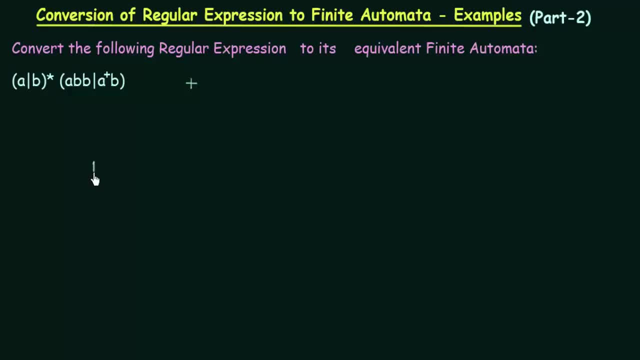 Its all closure. Okay, so let me take a state which I will call state number one And let me make this the final automata. Okay, so let me take a state which I will call state number one, starting state, and if you see that this is a closure, so whenever we have a 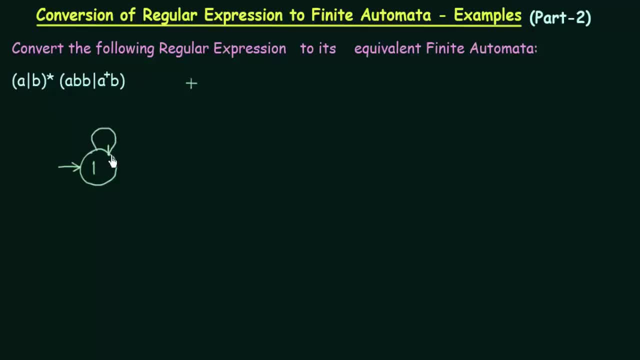 closure. what we do is we make a self loop. that is what we have studied. now, when will it go to this state on either a or B? so, on either a or B, it will go to this state one itself. okay. so now we have completed the a or B closure part. 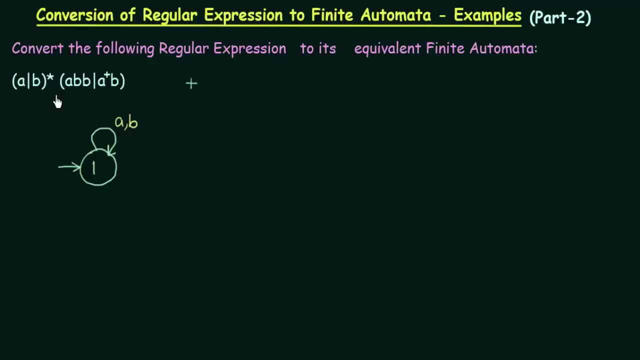 now let's come to this part. now. if you see here, you see that after this sequence it's like an end and it is followed by a BB, or a plus B, and this plus is not a plus in between a and B, but this is a plus over this a and we 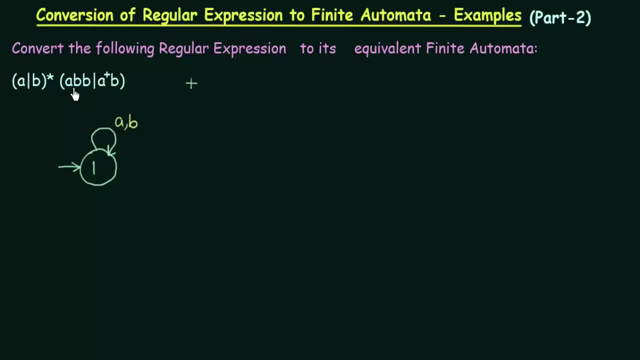 will see what it means. so first let's do this part a, B, B. so for that, let me make another state over here, which I will call state number two, and you can see that this is a closure, and this is a closure, and this is a closure. 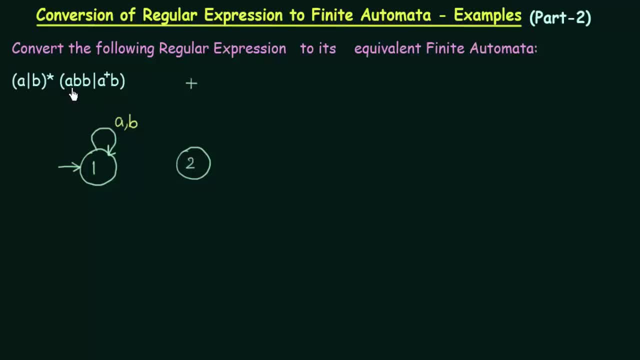 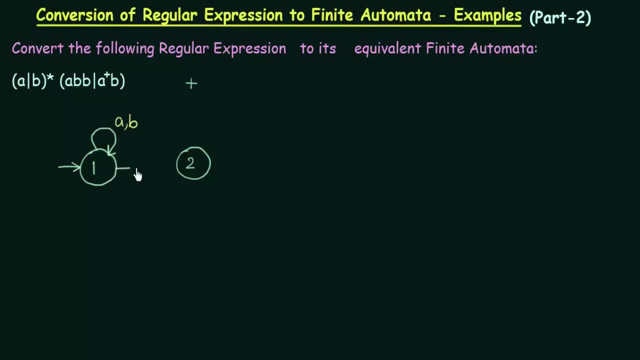 keep moving forward. so from here, this state 1 will go to state 2 on getting input a. that is this a over here, and then I will make another state over here, which is state 3, and I will send this state 2 to state 3 on getting input. 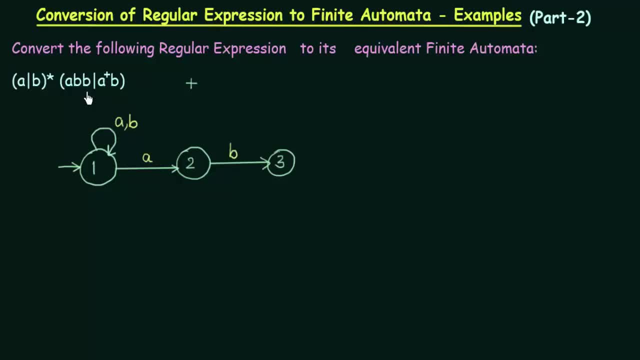 B, which is this B over here, and there is one more B for that. I will make another state, which I will call state 4, and state 4 will also be a final state, because this is a terminating symbol, and this 3 will go to state 4. on getting the. 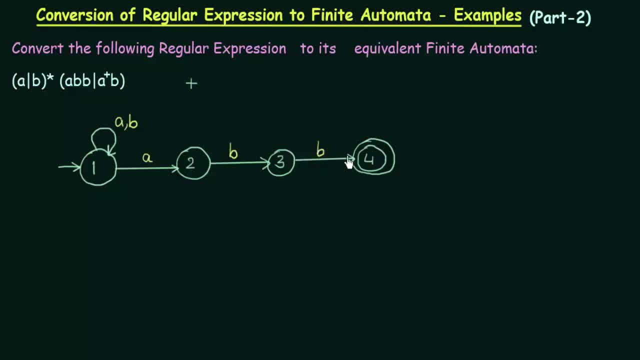 next input: B. now we have completed this part- a BB and, followed by this, we have an or symbol, which is followed by a plus B. now, whenever you have an or symbol, you have to continue from the state where you started. now here, this is the state from where we started this: a BB and since it is an or, this also will be. 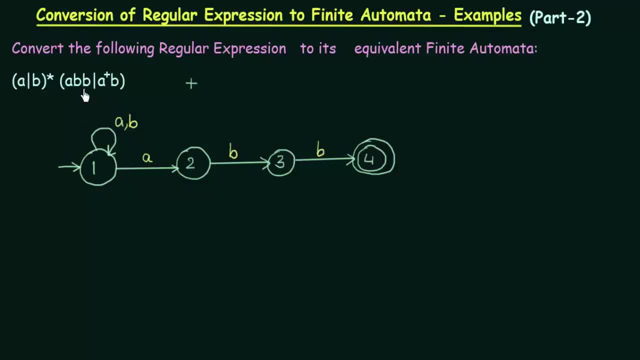 followed from this same state itself from where this was started. ok, so let me make another state here, which I will call state number 5, and I will send this 1 to 5. on getting input a. now we are going to design for this a plus. now, what is the meaning of this? 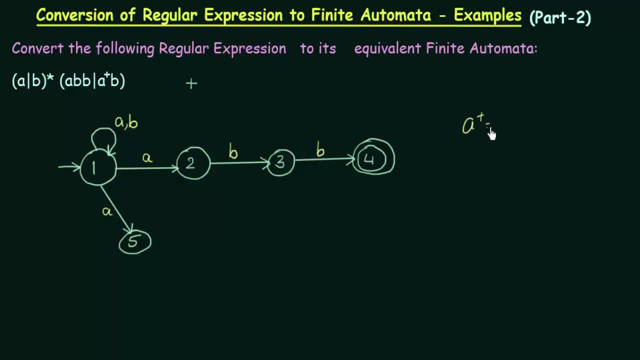 a plus. a plus. if you remember, when I taught you the identities, I told you it means one or more number of s, so it could be a AAA, and it would go on. now, what is the difference between a plus and a closure? in a closure, it can also include the empty symbol and followed by any number of s. so 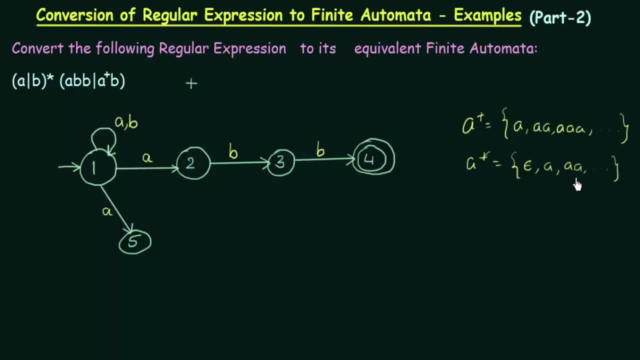 the difference is that in a closure there could be zero or more number of s, but in case of a plus it will be one or more number of s. that means at least one a should be present. so as we design for this a plus over here, what we do is, in this state, number five, I give a self loop and I put a over. 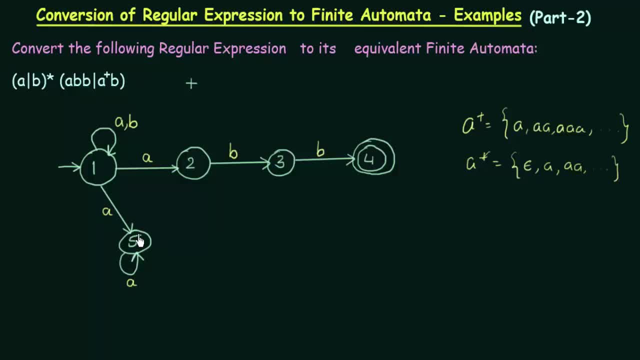 here now. if you look at this state 5, which is for this a plus, we see that it will come to state 5 only on getting at least one a. it will come at least on one a, and after that it could get any number of s. so we make sure that at. 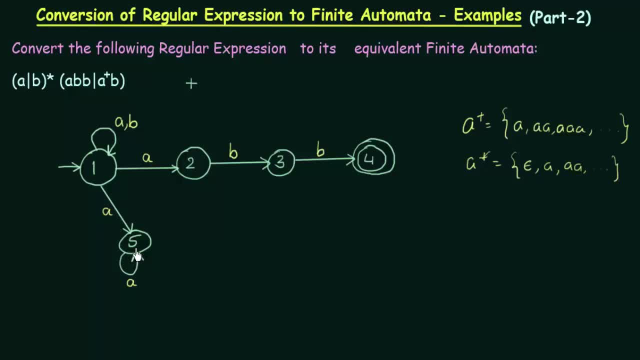 least one, a, will be present, followed by any number of S if required. so we have successfully made the automata for this: a plus. now it is followed by a- B. so there is nothing in between, it is just written together. so for it is be, i'll just make another state, which I will call state 6, and since that 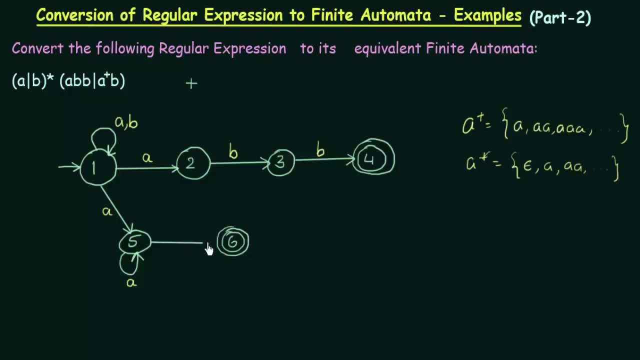 is also the ending symbol. so this will be a final state and this 5 will go 2. this state 6 on getting the input b. so that is for this one. so for this a plus we have designed this- and for this, for this b. here we have this part, so now we have successfully made the final automata.